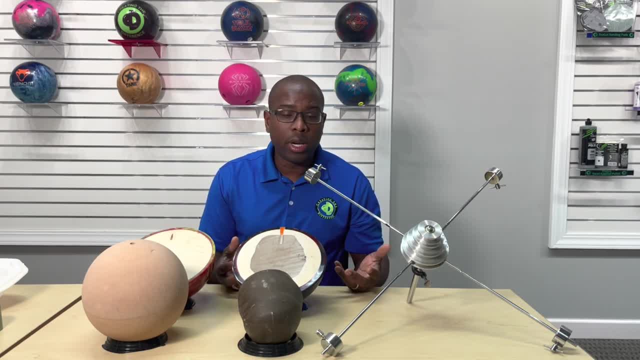 performance standpoint. How does that impact my ball motion and when do I need what? So I'm going to give you a visual example Of kind of what that means: High RG versus low RG. I'm going to use this device right here Now. these. 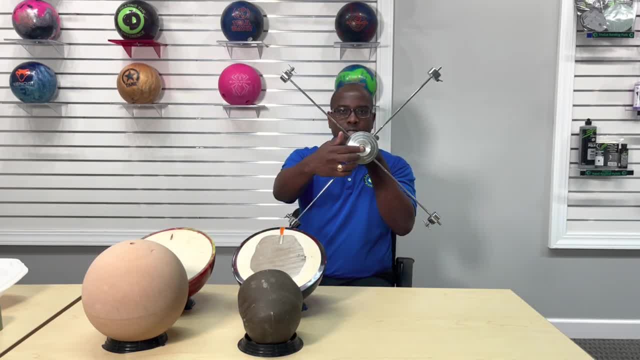 have weights and these weights are away from the center of the piece, So this would be like the center of the core shape. This would be the center of the core shape here and this is the mass. So in this particular orientation, we have the mass in what's considered a high RG location, because it's 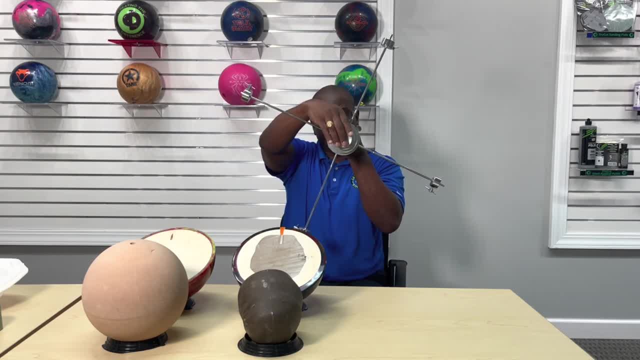 farthest away from the center, of the core, center of this piece, this bar right here. So as I spin it, you'll see as it spins, it spins kind of slow And that's just a little bit of a way to function of the mass- is far away from the center, like the bowling ball that I showed you, that is. 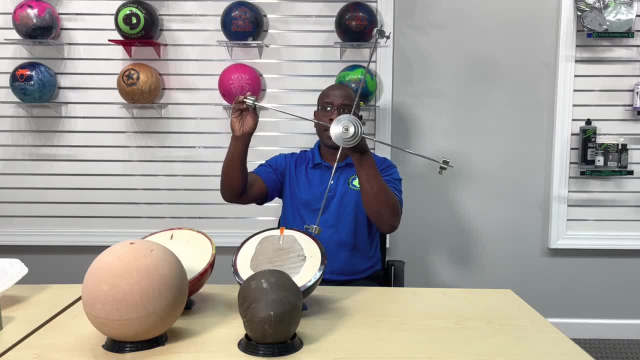 actually right here. This would be a high RG configuration. Conversely, as I take this mass and begin to move it in, I'm moving it more toward the center here, more toward the center of the core shape, more toward the center of the axis here. What that's going to allow me to do is I'm going to 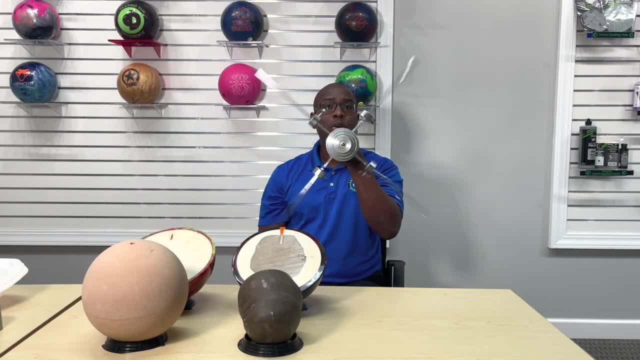 then apply. you know about the same kind of force. not much, but you can see it's spinning a lot faster, And that's because more of that mass is concentrated more toward the center, which will increase the rate at which the object, in this case this device, wants to rotate. Now you say, well, okay. 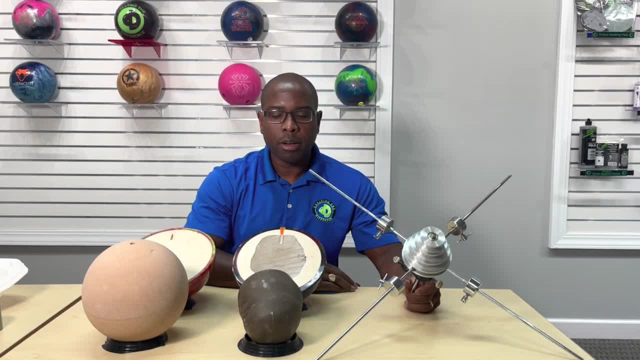 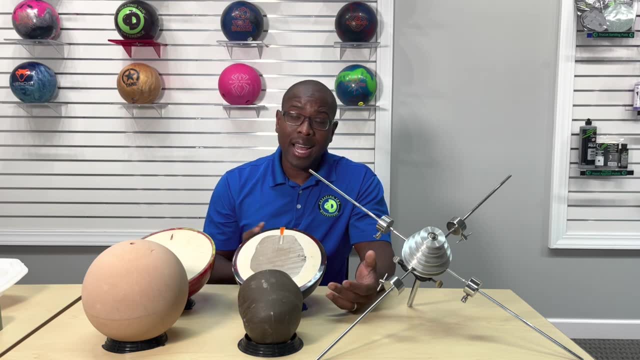 that's great, Ron. How does it help me as a bowler? When do I use these? Does it matter? So what I'll tell you is this: If you are bowling on a condition where you've got more oil and you need your bowling ball to kind of pick up a little bit earlier, more like a low RG core shape would. 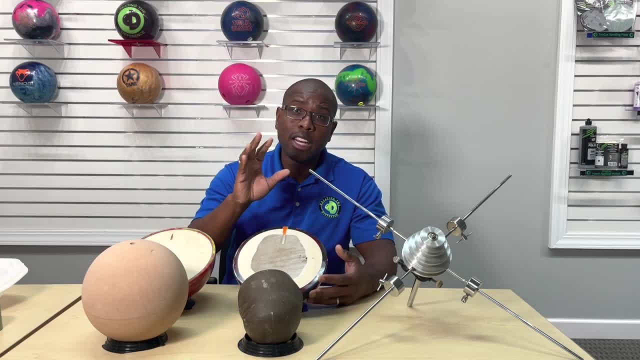 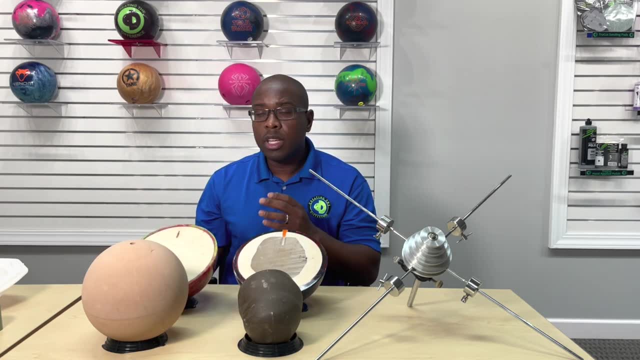 be your choice. If you're bowling on drier lanes and you need the bowling ball to get down a little bit further, more like high RG bowling ball would be the choice. Now, obviously, there's other things that go into this. The cover, stock, the surface, all those things matter as well, But strictly from a core standpoint. 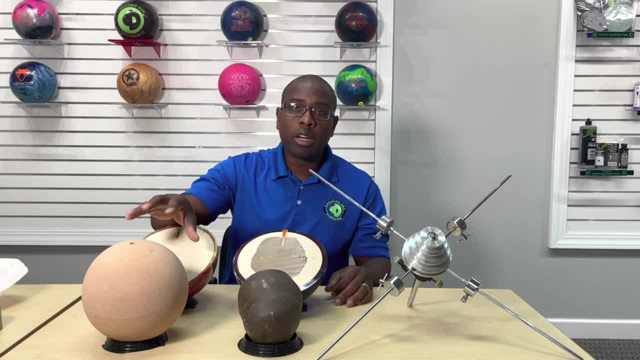 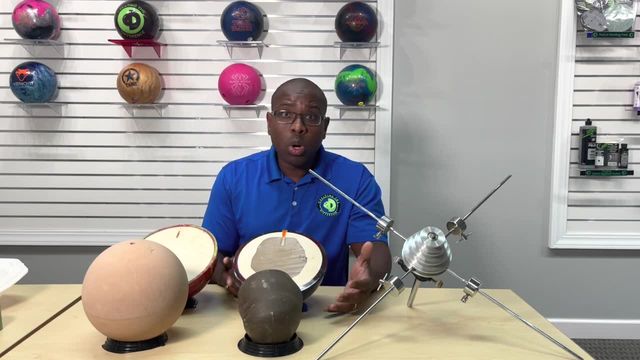 low RG cores tend to roll earlier. high RG cores tend to roll later. That's just kind of, in general, what happens. So now you've got some more information about RG and kind of what they do and when you may want to use which one. If you have more questions, feel free to join our staff. Just.